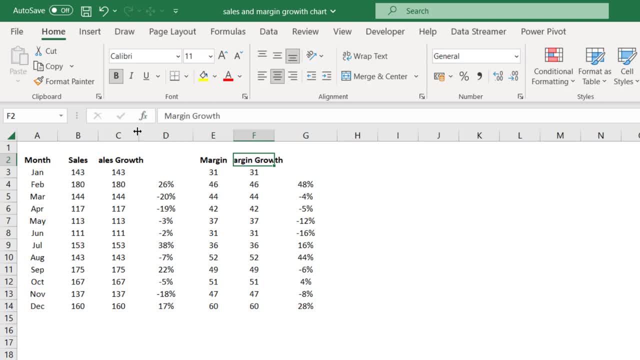 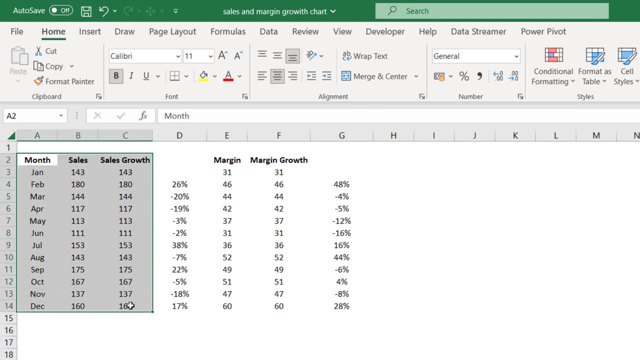 from column G to column F. Now, this is not an error. We're going to create the chart that we are looking for. This is, in fact, an interesting chart trick that a lot of professionals use, and you will soon understand when you follow along in this video. Select all these columns: A, B, C, E. 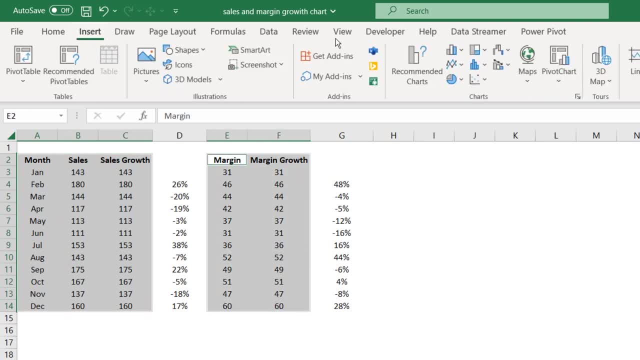 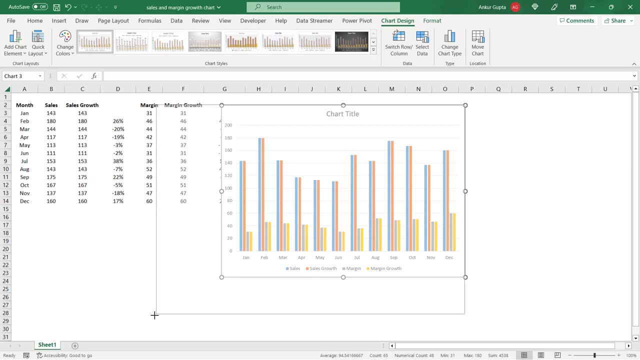 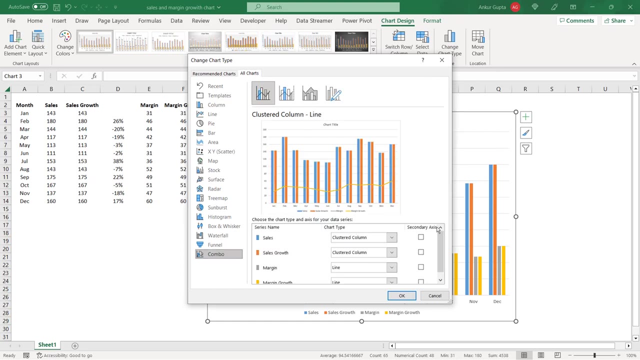 and F and let's insert a chart on this data. Go to insert. choose a 2D column chart. Now, this is not the final output. We're going to make a lot of modifications to this chart to get the desired output. First, go to change chart type. click on the combo option here. 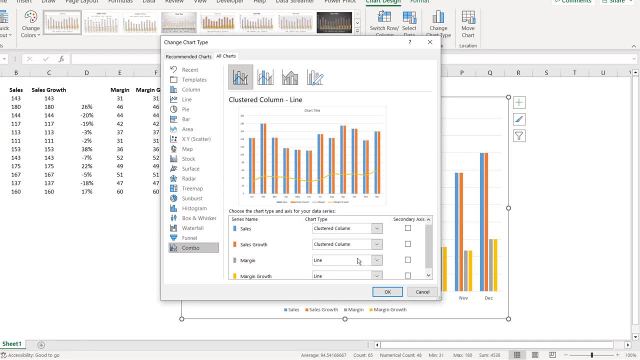 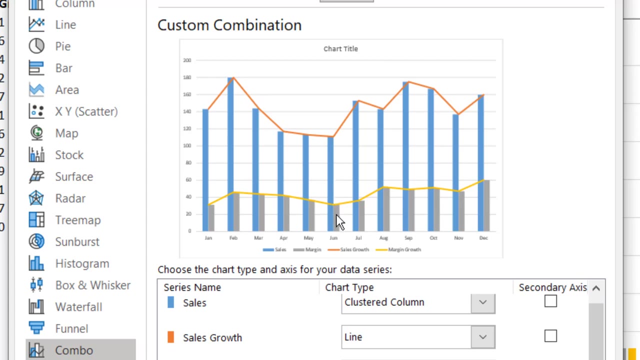 and change the chart type of sales and margin to column and the other two to lines. So if you look at the chart here, you observe this blue column represents sales and the gray one represents margin. Now if we plot them like this, adjacent to each other, then this: 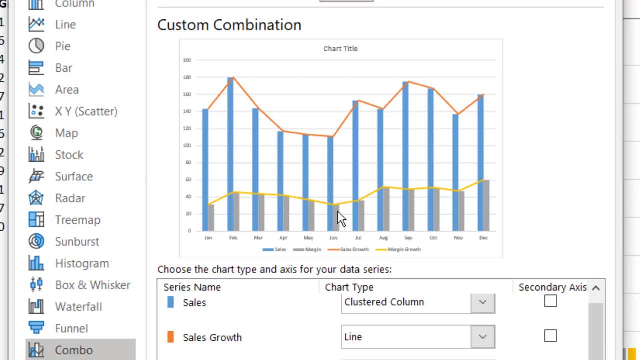 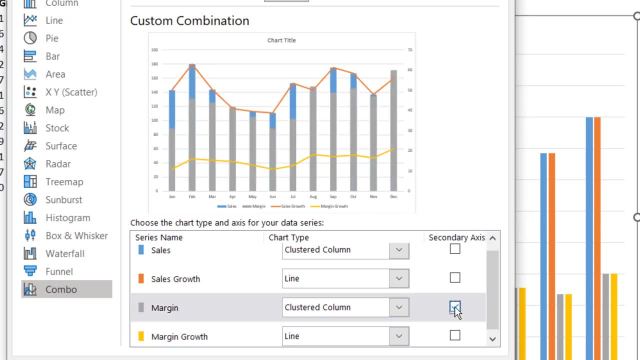 occupies a lot of space in the chart. So in fact we're going to put the gray column over the blue column here. Secondary lenses Also. we need to take both the lines which represent growth also to secondary axis. Now click on okay And you have a chart which looks something like this: 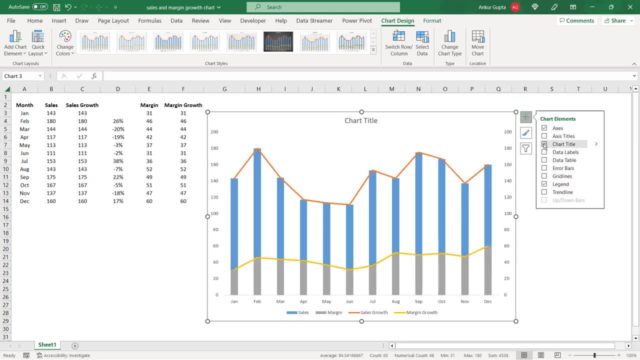 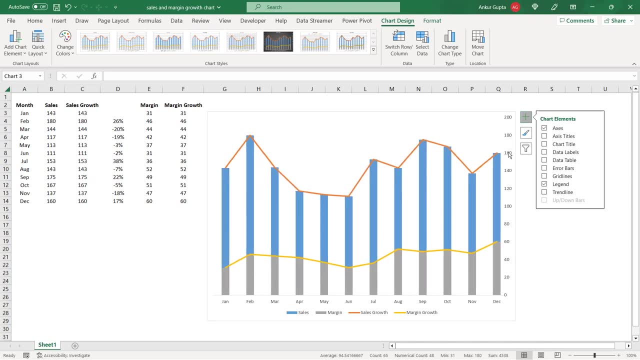 Now let's remove the grid lines and the chart title to save space. Let's also get rid of the vertical axis, the primary as well as the secondary. Add data labels. So now the interesting thing starts. you observe the blue column and the orange line here. 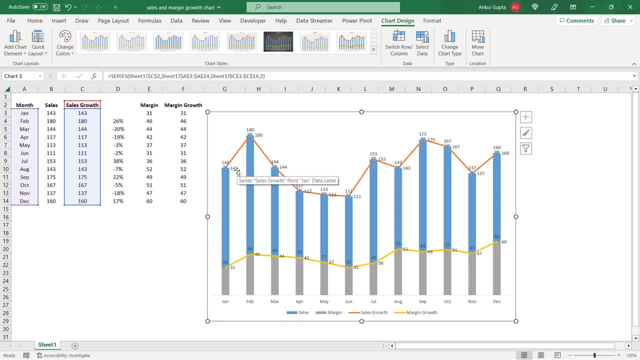 here represents sales. So we have the sales values in data labels twice: once for the blue column and second for the orange line. What we are going to do? we are going to replace the values in orange line from the values in column D. Keep following. click on the. 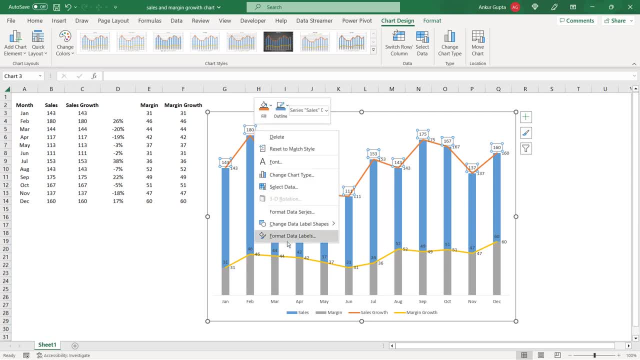 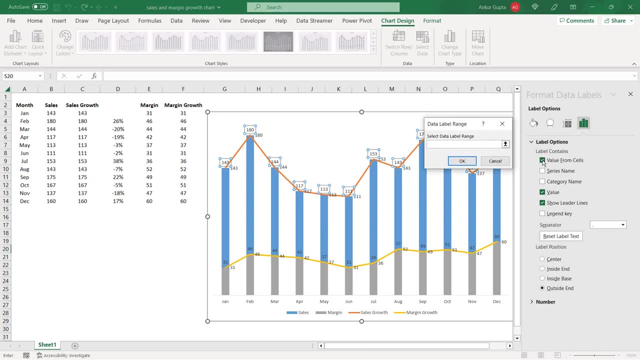 data labels here and now. right click and go to format data labels. Go to the last option here, which says label options, and click on value from sales. Now, here you can change the data label values by taking them from any part of your worksheet. So let's select. 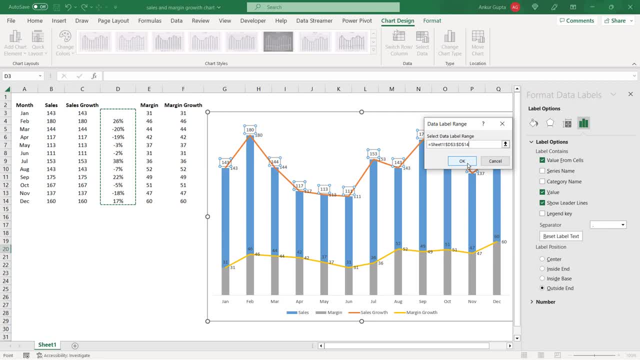 the values from column D. click on ok, and now you see, alongside the sales values you also have the growth values here. We do not want the sales figures to appear twice, so uncheck the value option here And you are only left with growth values. Now you might. 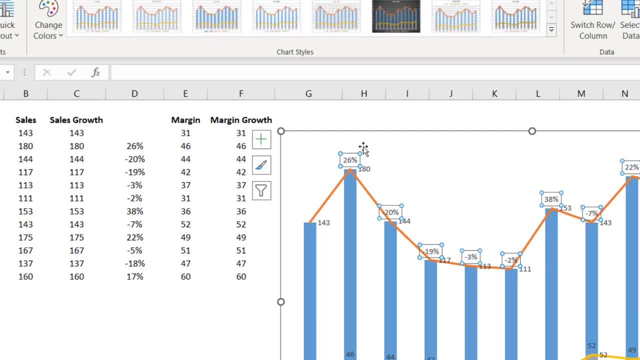 understand that why we took sales values in column C. this is because we wanted that the sales growth numbers should be the same as the values in column D. This is because we number should appear just over the sales column and this can happen when both the blue column 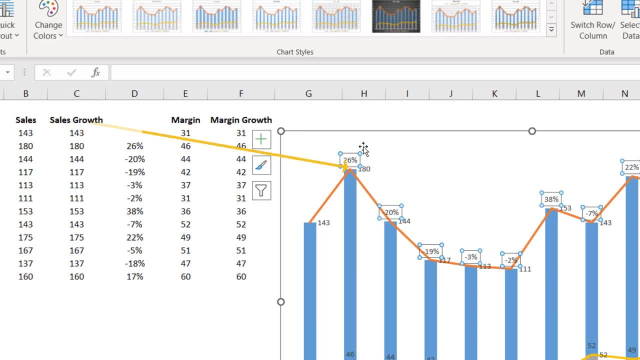 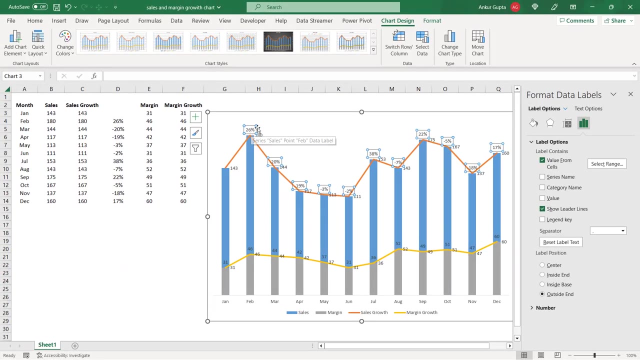 and the orange line meets at the same point. This point here represents 180 for the blue column and also for the orange line. So we need to plot our growth numbers just on top of the column, and this can happen this way only. We need to repeat this process for the margin also. 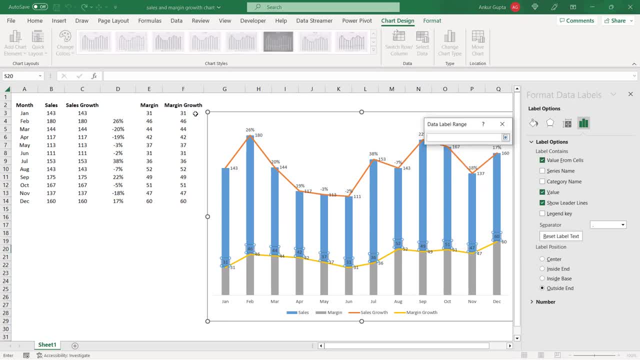 So click here. choose values from sales. select the values in column G. Column G is actually hidden here, but it does not matter. we can still select that and now click on ok and you have the percentage margin growth here. So we are very close to the final output, but we need to make some modifications to this. 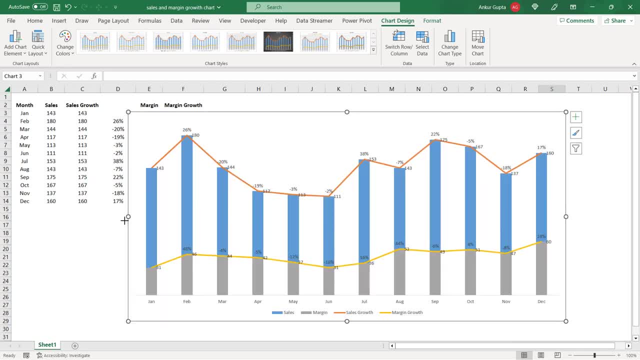 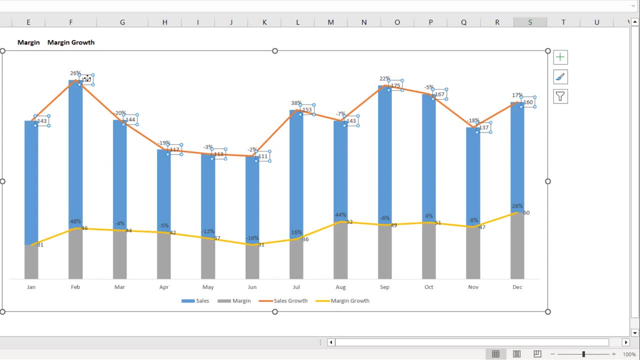 chart so that this becomes more readable. Right now, all the fonts and the colors inside the chart are not that appealing, So first of all, let's bring these data labels away from the other labels. so click here, go to format data labels, bring them below and repeat this for the gray series also. 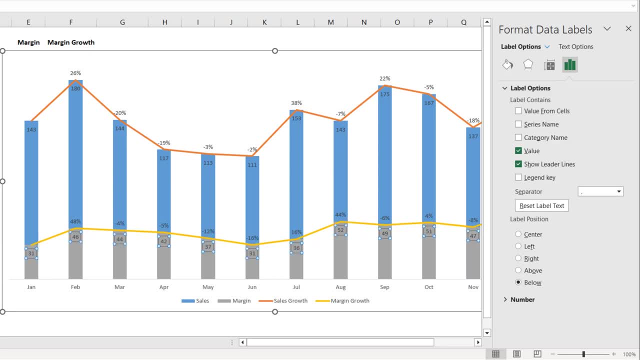 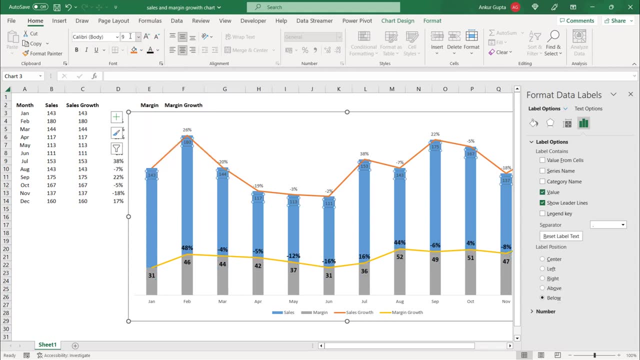 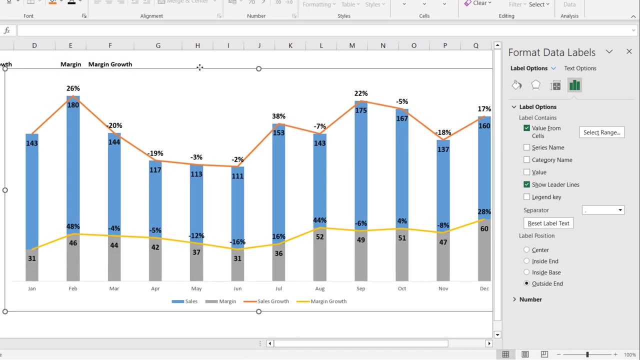 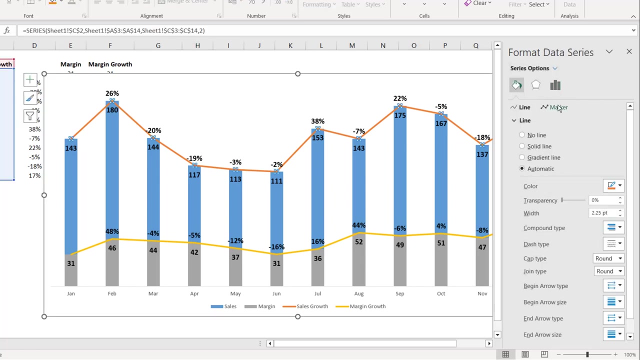 bring them below the other data labels. let's increase the size and font of the data labels so this looks much more readable. now we're going to insert markers on the orange line. so click on the orange line, go to the series fill options, choose marker marker options, and you can choose any pre-designed built-in market template. 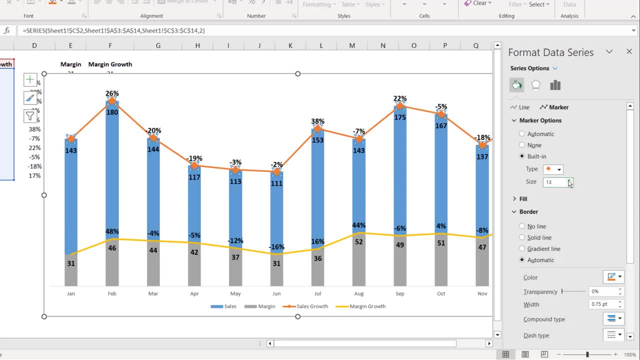 here. let's choose this one, increase the size, and you have something like this appearing here. let's repeat this for the other labels. repeat it for the yellow line also, which is for margin growth. this time let me take another shape type, so this brings a beautiful artistic effect into the line. 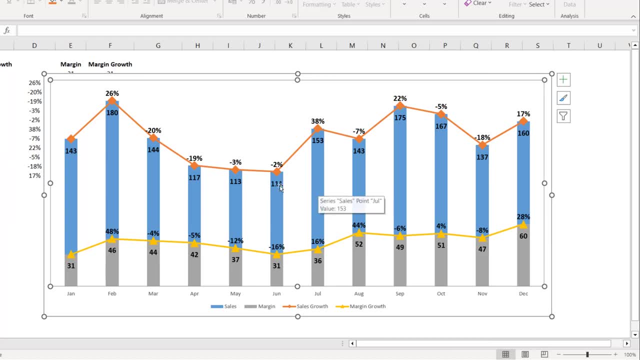 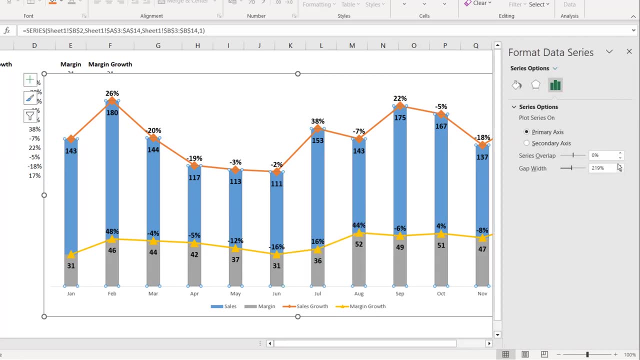 charts, we can change the colors of all the series so that our font and the series colors do not merge with each other. so click on this data series and now I'm going to choose a fill color of a light pink shade. you can put this code here: 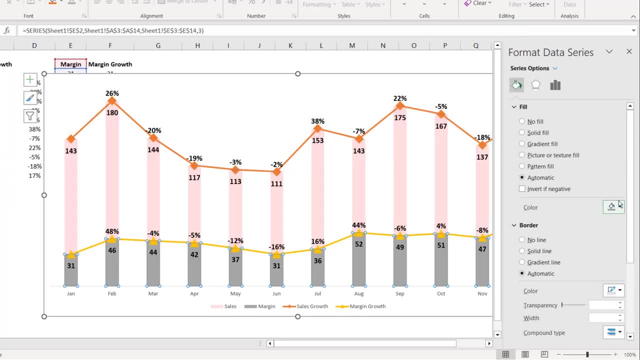 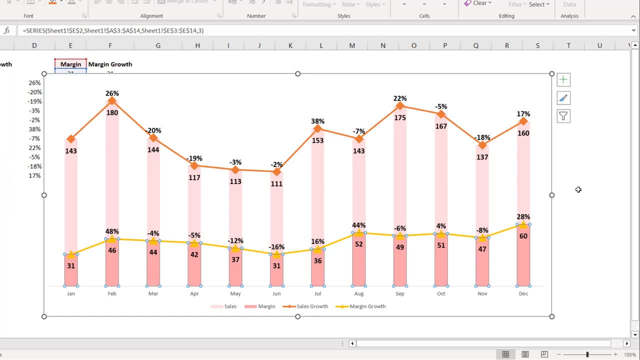 click on ok and here you can put this code. but there are a lot of other options also in the format, data series and data labels menus, which you can experiment at your end and you can make this chart as beautiful as you want to. so we have our chart ready and we have 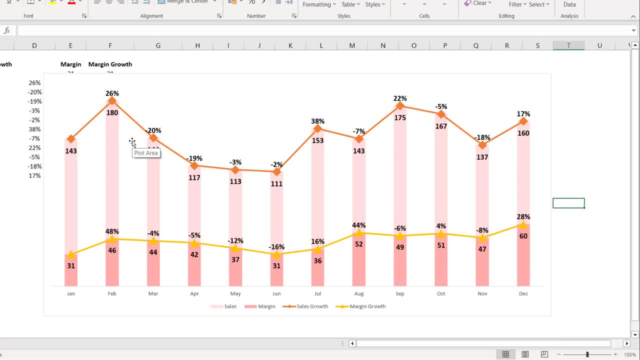 four parameters on four different charts, plotted together in a single chart, and all of them are easily readable here. now one important thing: we actually have a hidden parameter, which is a fifth parameter in this chart, and that parameter is margin percentage. so where is margin percentage? we do not. 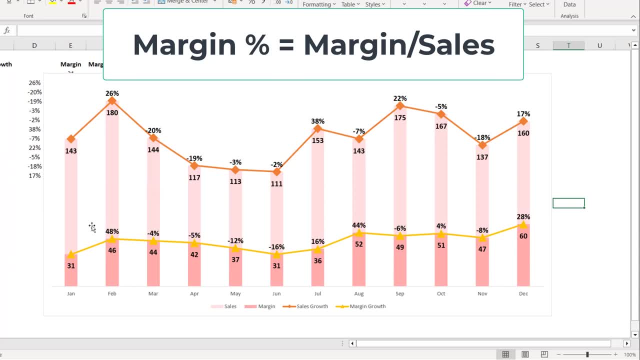 have the exact numbers plotted here. but if you look at the January figure- let's not look at the numbers- but even when you look at the colors here, you observe that the dark pink color almost occupies 1, 4th of the light pink column. so this: 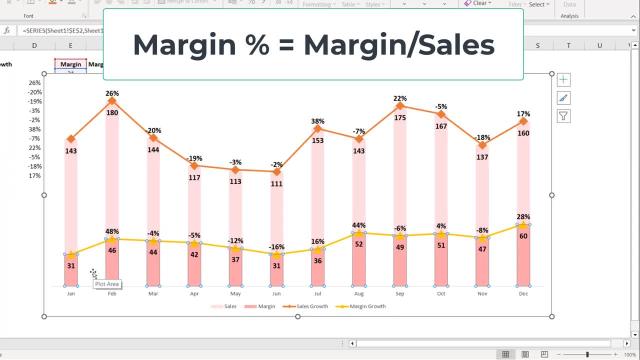 means our margin is roughly around 25% or, on the safe side, between 20 to 30%. so this can give you an idea, if not the exact number, for our fifth hidden parameter, that is, margin percentage. so I hope you're able to understand this chart now. so when you compare January to February, this means the sales increased. 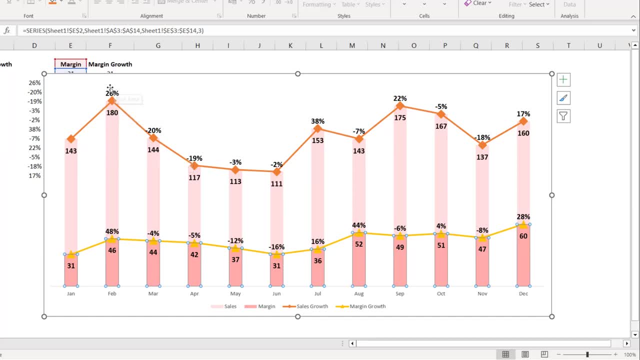 from 143 to 180, which was an increase of 26%, and similarly for the margins also, the margin increased from 31 to 46, which was an increase of 48%. now this chart is very important and if you want, you can take it several levels above also, suppose, instead of just having one. 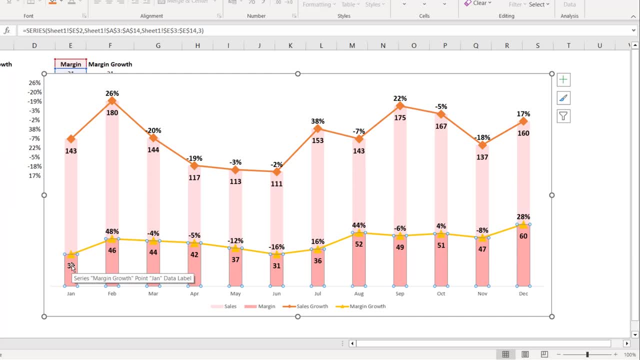 margin. if you had two margin figures, one for the gross margin and other for the operating margin or the net margin, then you can put three columns here, one light pink, one a middle shade of pink and the third one a dark pink color, and similarly you can have three lines also, and still this chart will be equally. 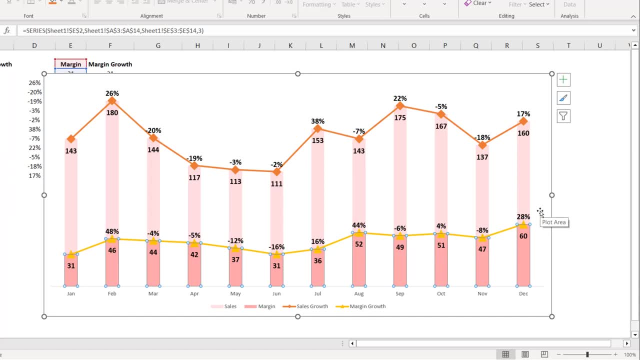 readable. so that's it for this video. to watch more such videos and to take your Excel skills to next level, consider subscribing to my channel. watch all the latest videos that I keep putting in, also the videos that I have already put on my channel. increase your knowledge, become. 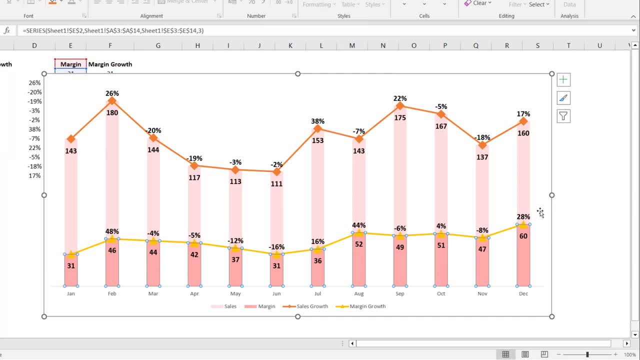 professional in Excel. so thanks for watching this video. have a nice day. 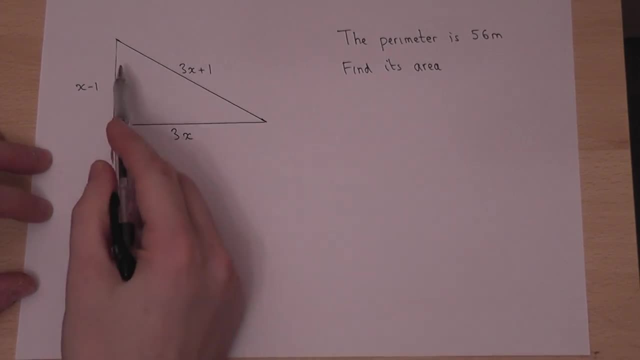 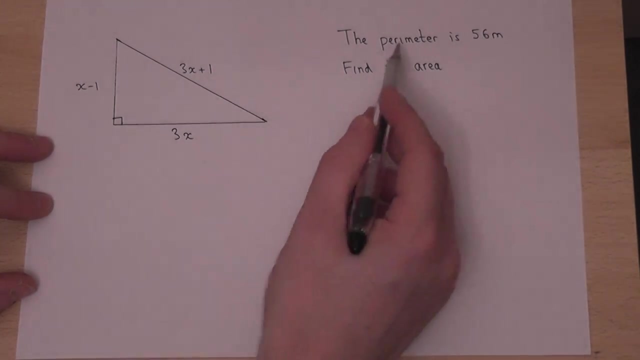 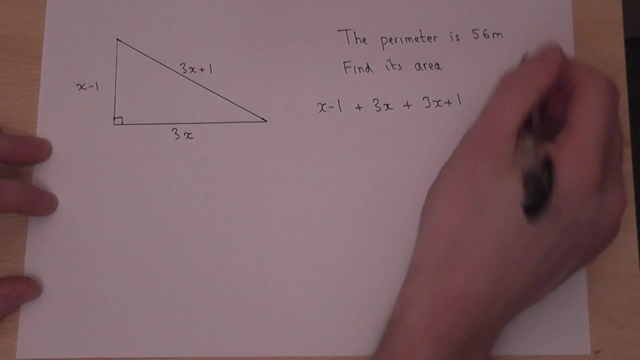 This question involves algebra and a shape, and we're told that its perimeter is 56 metres and we're asked to find its area. Now, the method here is to write down an equation involving the perimeter. Now, perimeter means add together the sides, So we therefore know that x minus 1 plus 3x plus 3x plus 1, that side, that side and that side must equal 56. 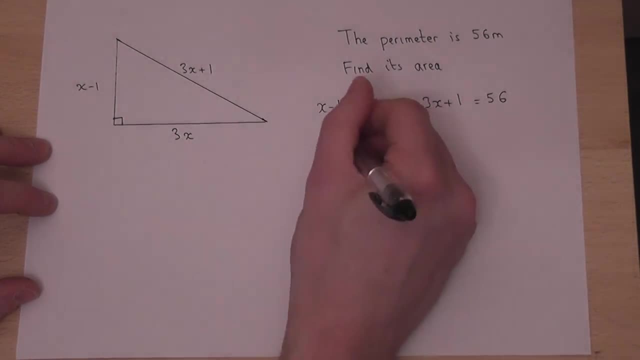 If we make this simpler: x, 3x, 3x is 7x minus 1 plus 1, they cancel out. so 7x equals 56. So x just equals 56. Divided by 7, which is 8.. 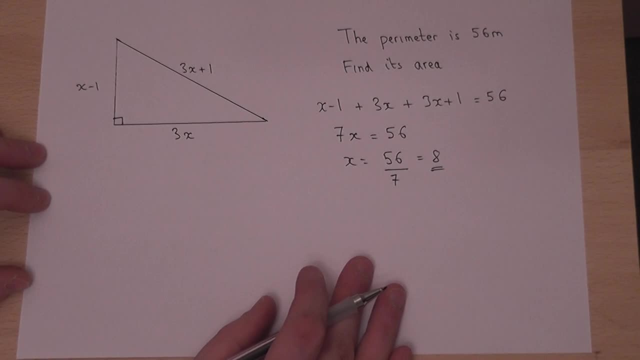 So we know the value of x. We can therefore find out the length of the sides 3 times x must equal 24.. x take 1 must equal 7.. And also 3x plus 1 will equal 25.. So these are the dimensions of. 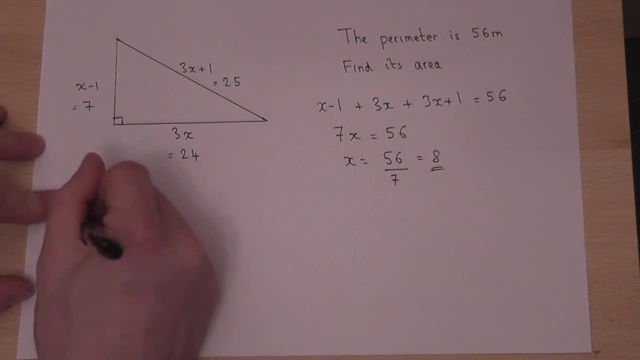 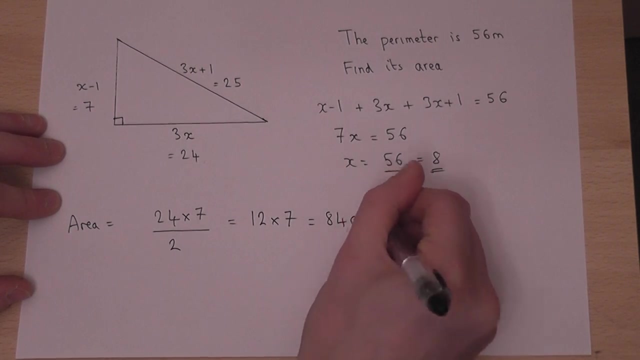 the triangle. And to find the area, we just have to work out a half of the base times, the height. So the base times by the height halved. Well, a half of 24 is 12.. So 12 times 7, which is just 84 centimetres squared. 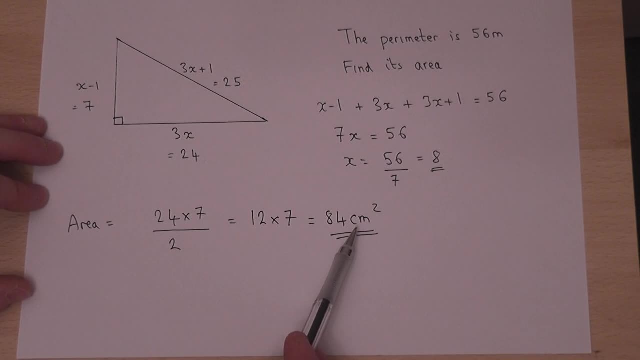 So the area of the triangle is 84 centimetres squared. We loudly give this requirement. Sorry, I fingerpicked the fallback. It should have been a minute ago And then they meant to say it should be a minute. we take the product. and they said so. these values are 22 and zero, which is joint. Instead of difficulty jewel, it's just currently Number 2.. What are these values actually equaled to? Well, let's start with 2.. So x, 3x.